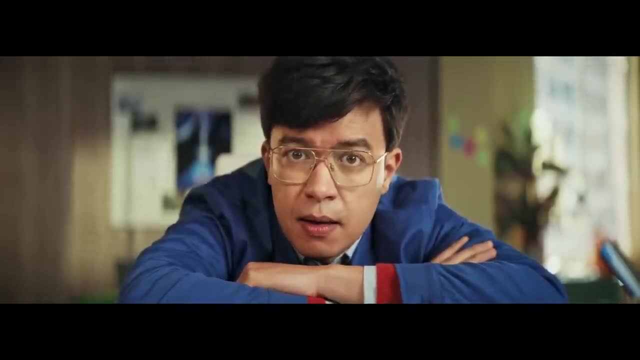 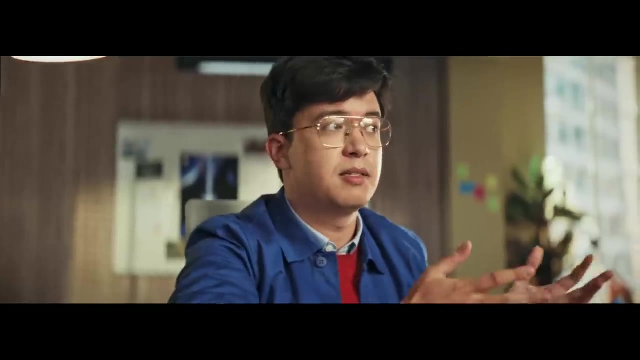 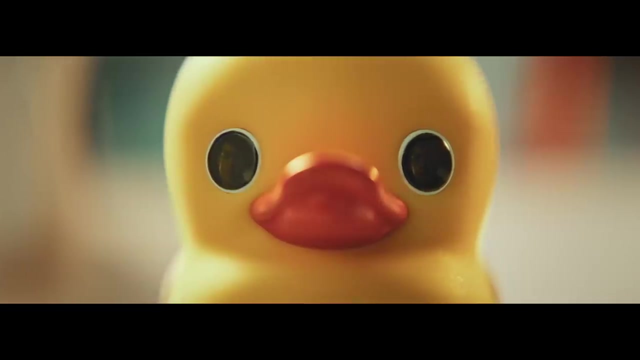 What do you mean? what is GitHub? It's the largest, most complete development platform in the world. Millions of developers use it. And it's not just developers: These days, every company is a software company. I thought you might say that. Come on, let me show you. 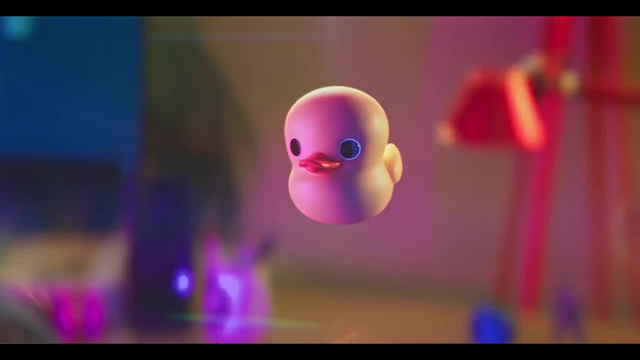 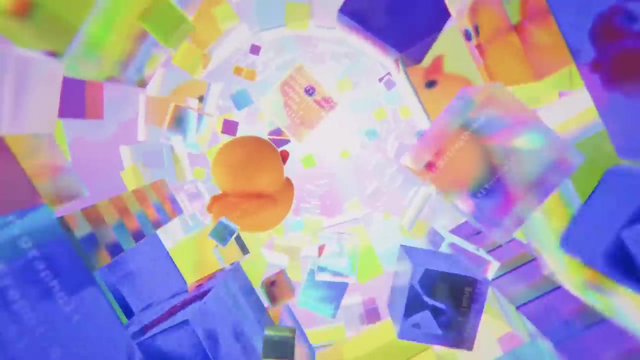 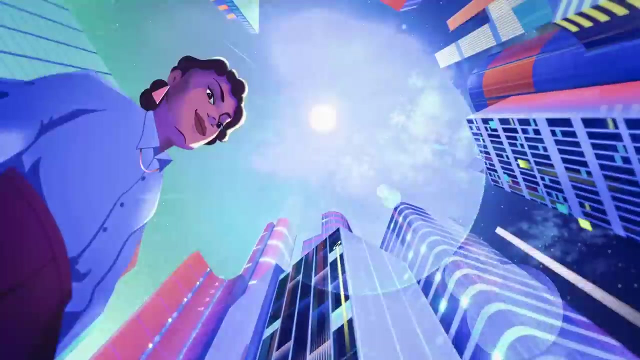 GitHub is an enterprise-transforming, startup-launching, community-driven, super-secure, open-source-championing cloud-based platform. It's where the world builds software. We created algorithms And global businesses. We even went to Mars, Or at least our code did. 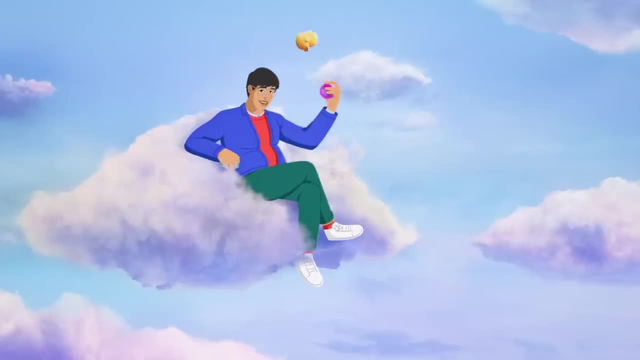 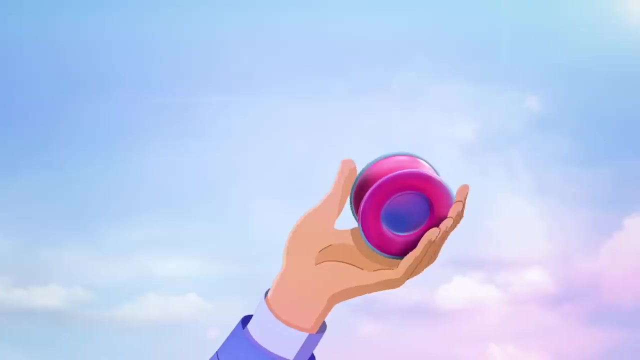 Oh yes, With GitHub anything is possible. But how Say? this is Sanal, a senior software engineer And this is a team's project on GitHub. Sanal and her team can create their own branches of code to work together in parallel. 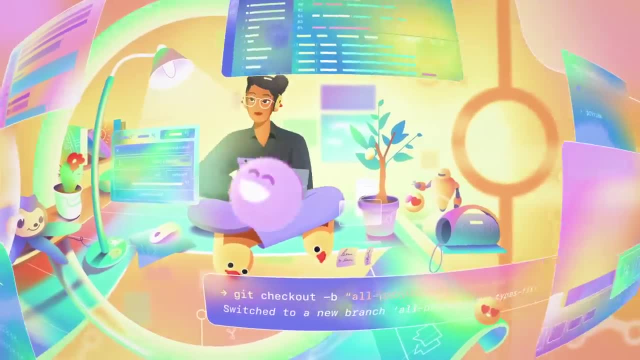 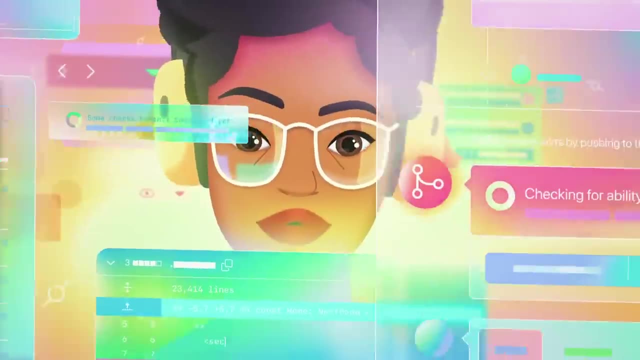 This is my branch, An alternate timeline where I can build, squash bugs and safely experiment. There are communication and task delegation tools right next to my code, So when we're ready to merge, we merge Instantly. It works with thousands of branches for over a million years. 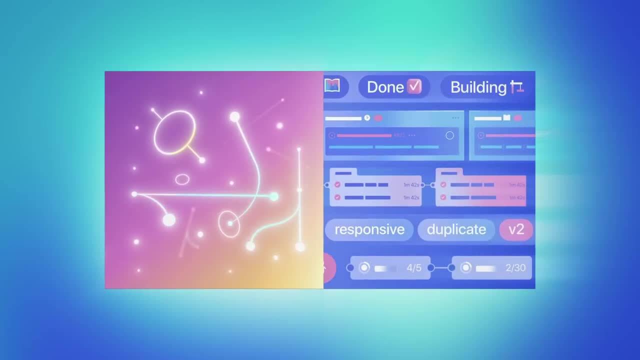 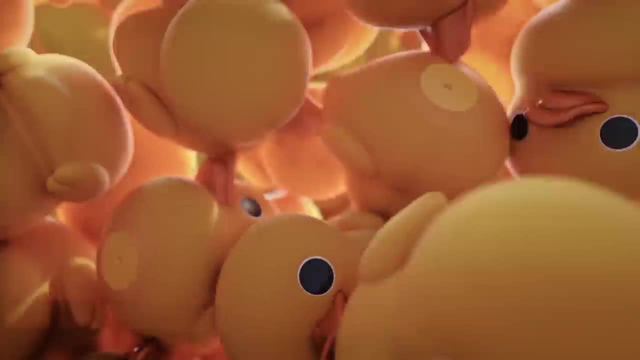 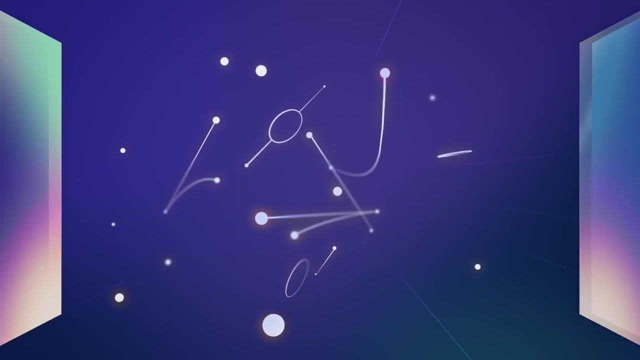 And with built-in project planning automation, CICD and AI-enhanced code editing at every step. You can move fast and get your ducks in a row, But we gotta be safe about it. GitHub has advanced security with automatic vulnerability detection, secret scanning and more. 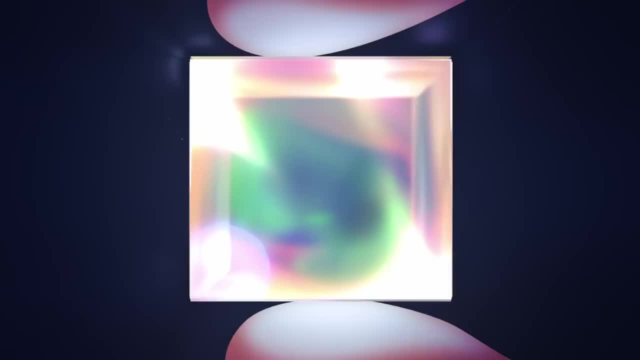 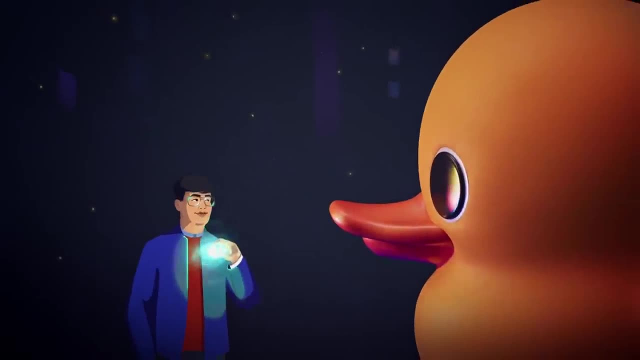 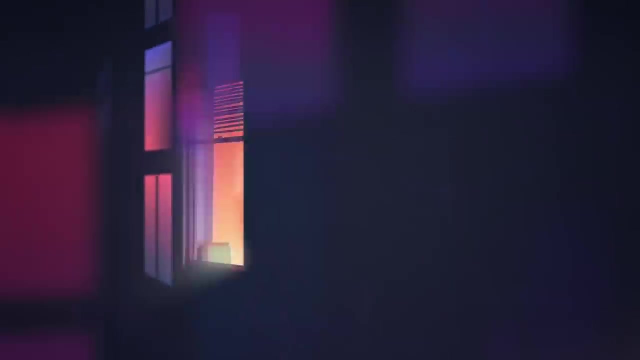 So we can build and ship safely And securely. So now you know what GitHub is. you might wonder who GitHub is. It's a student learning to code. It's disruptors revolutionizing music. It's a CEO transforming a global company.